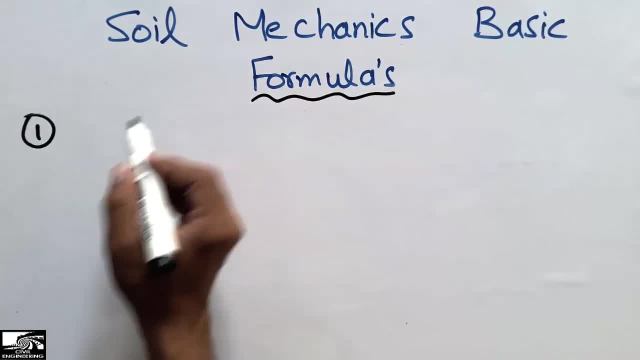 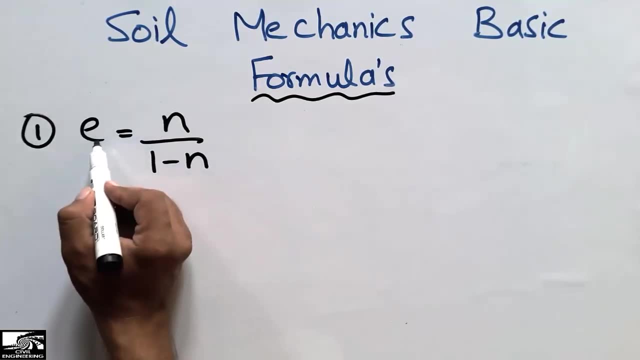 The first formula which is used in the soil mechanics is: the E is equal to the N divided by the 1 minus N, Where E is the void ratio, N is the porosity. So these are the two different terms here used in this formula. 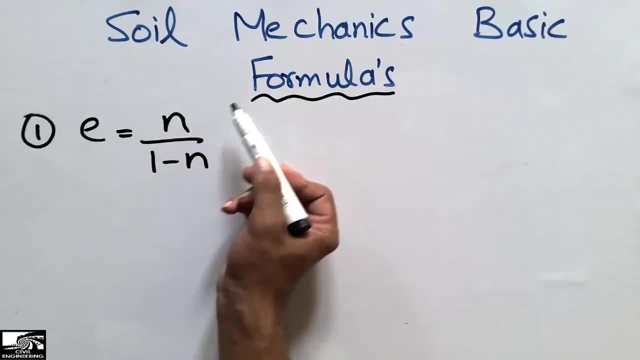 So if 1 is known to us, If the porosity is known to us, then we can find the void ratio. Now the second formula is if we are given with the void ratio, so we can find the porosity by this formula. 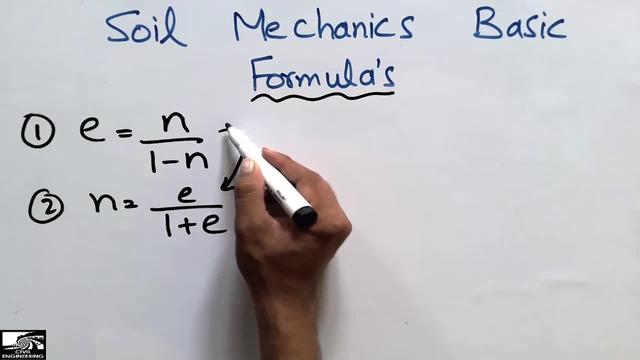 So this formula can also be derived from this formula. These formulas are interchangeable. So the third formula is that the S dot E is equal to the W into G. This is also mostly used in the soil mechanics, Where the S is the degree of saturation of the soil. 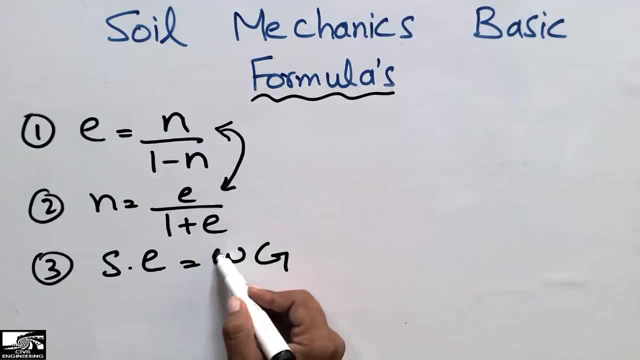 E is the void ratio of the soil, W is the water content And G is the specific gravity. So this is the formula, So we can find if we know the three parameters. For example, if we are given these three parameters. 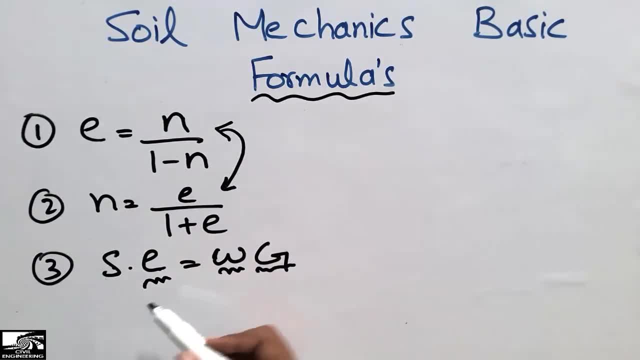 So we can find the degree of saturation If we are given with these three parameters, we can find the specific gravity and so on. So this is also really used in the soil mechanics. The fourth one is that the gamma B, which is called the bulk unit weight. 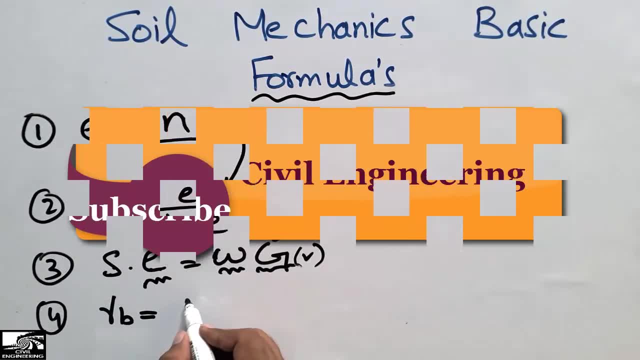 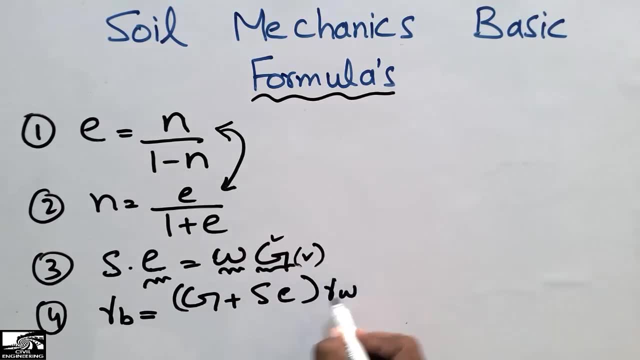 The bulk unit weight. there is some formula of G plus S, E into gamma W with the 1 plus E. Here we know that the bulk unit weight is equal to the. G is the specific gravity of the soil Plus degree of saturation into void ratio. 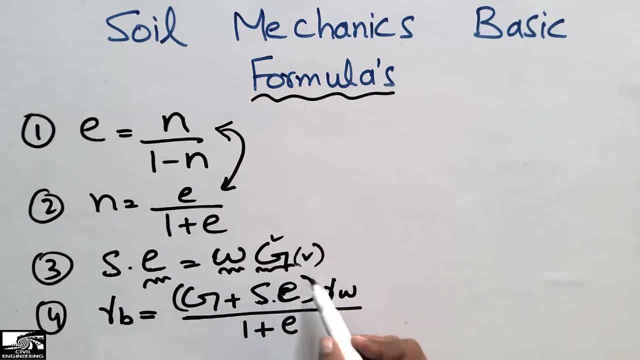 It is multiplication here. These both are multiplied in the bracket And then the unit weight of the water. This is the unit weight of the water- This is not the same as the bulk unit weight- And then divided by the 1 plus E. 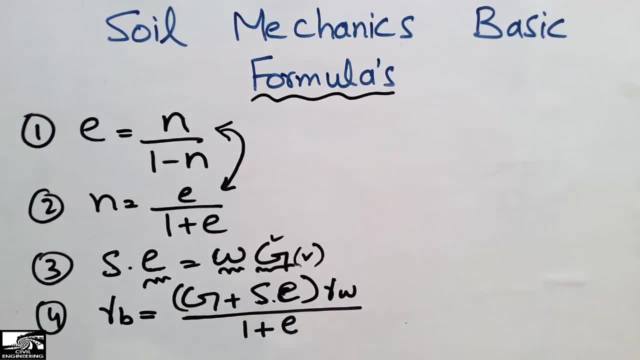 So we can find the bulk unit weight by this formula. And the bulk unit weight is also equal to the total weight of the soil divided by total volume. We can find the bulk unit weight by this formula. But in some problems we are given with the sum of the parameters, like these ones. 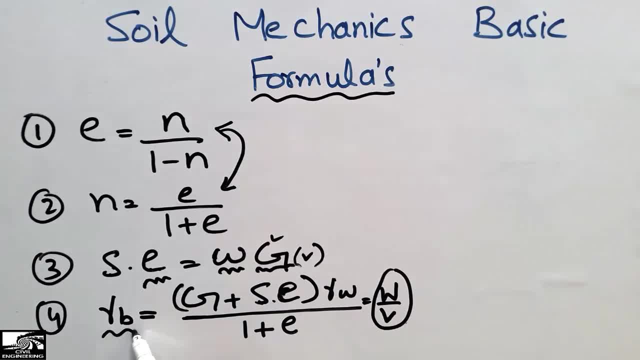 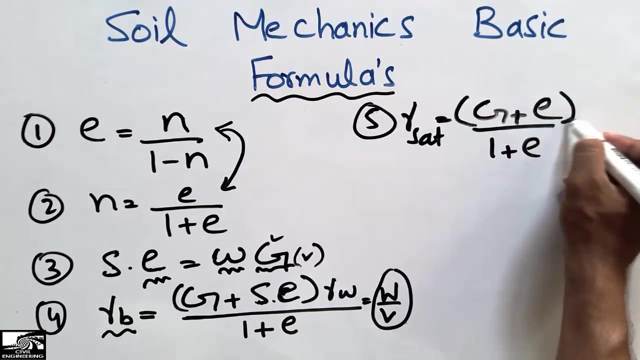 So we should know how to find the bulk unit weight by this method. So the fifth formula is used in the soil mechanics. It is the gamma saturated. It is equal to the G plus E divided by the 1 plus E. Here again, gamma W. 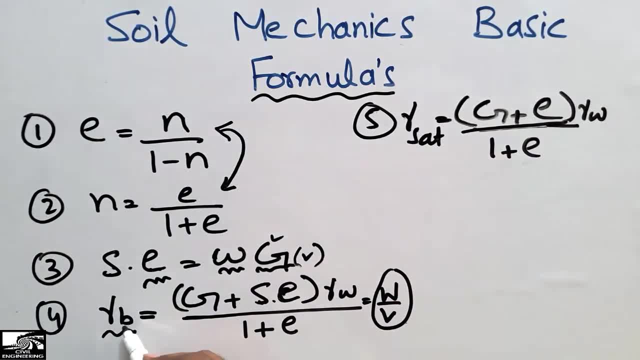 The only difference between the gamma saturated and gamma B, which is bulk unit weight, And the gamma saturated difference is that here S is used and there is no S, Because in the gamma saturated case we have degree of saturation is equal to the 1.. 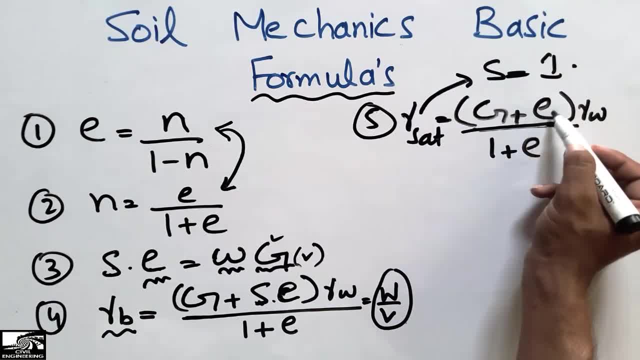 So we place here the 1.. So this is now called as the gamma saturated. The only difference, the only we can learn this formula if we learn already this formula. So this can be easily learned just by removing the S. 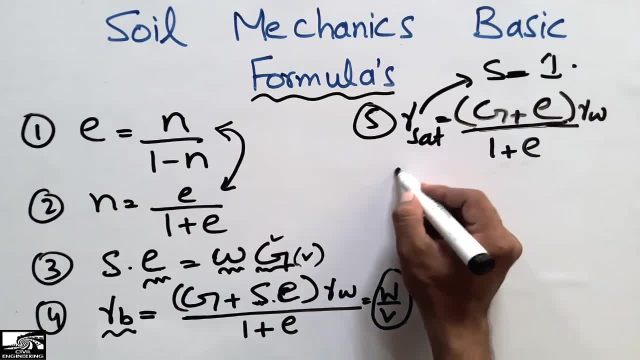 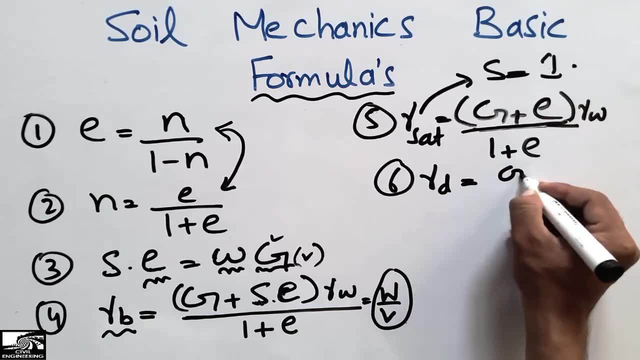 Because S is 1 in case of the gamma saturated. Now the sixth formula is the dry unit weight. Gamma D is equal to the G into gamma W, which is the unit weight of water divided by the 1 plus E wide ratio. 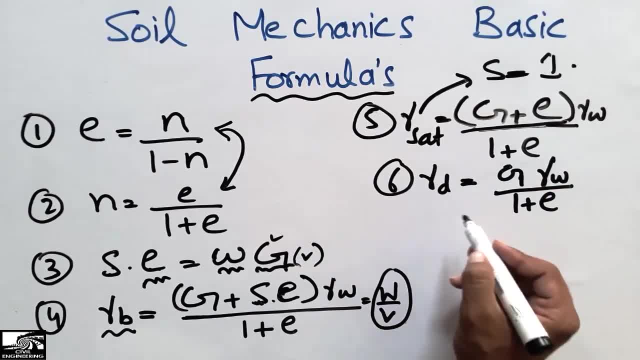 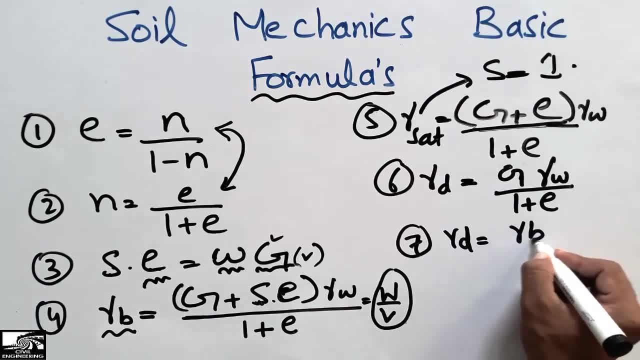 So this formula is used to find the gamma D, which is the dry unit weight of the soil. The seventh formula is also for the dry unit weight, but in terms of the bulk unit weight Right, 1 plus W. So this formula is also used to find the 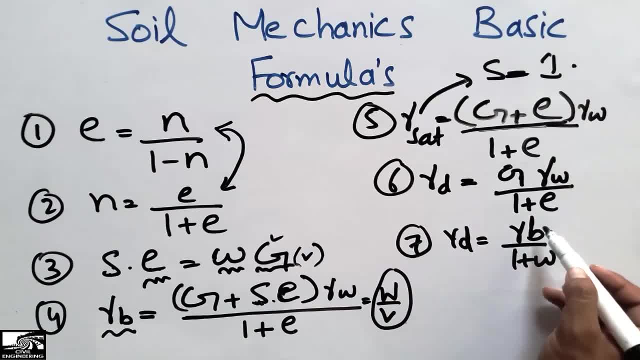 gamma, the dry unit weight of the soil. if we are given with the bulk unit weight of the soil by dividing the 1 plus in water content, The eighth formula is is that the gamma submerged. gamma submerged is equal to the G minus 1,. 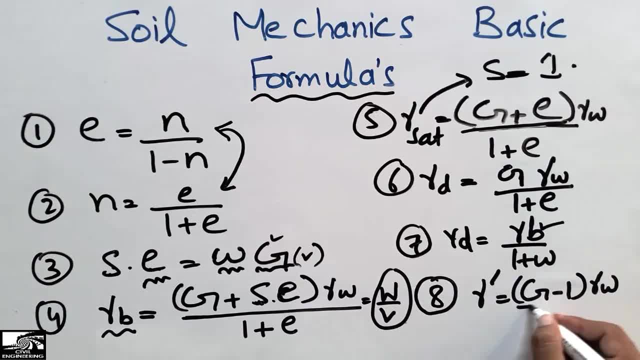 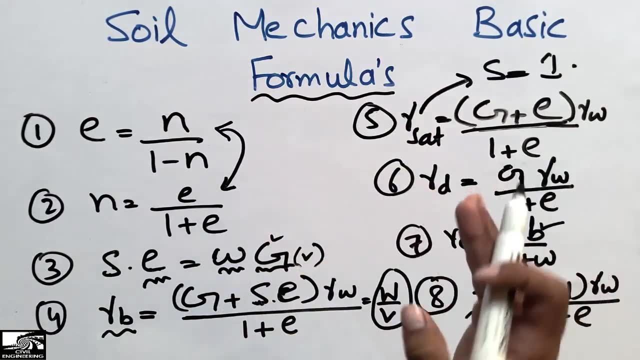 and bracket. and gamma W unit weight of water divided by the 1 plus E is the wide ratio. So this formula is used to find the gamma submerged. So these were the eight basic formulas of the soil mechanics. When you are going to learn the soil mechanics basics,